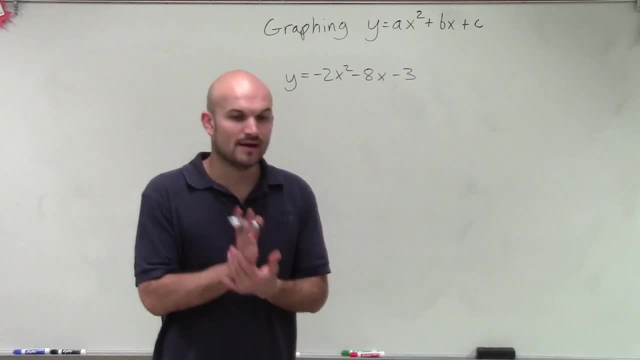 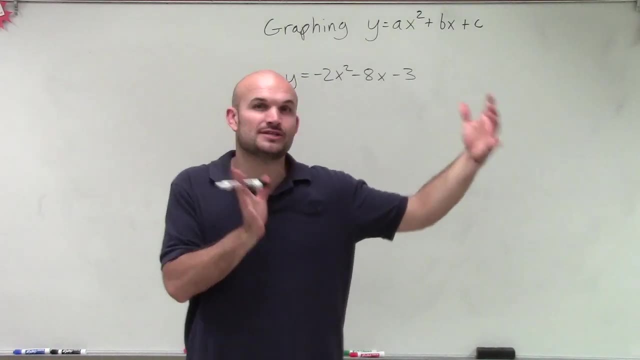 shown a lot of examples of choosing points to the left or to the right. what we notice is the y-coordinate to the left and to the right are exactly the same. So what I'm going to do now is let's just choose two points, either to the left or to the right, and then 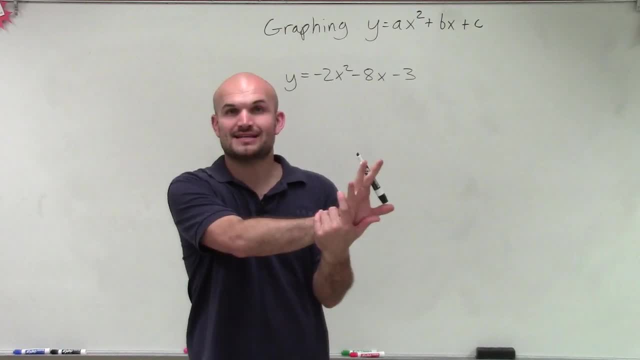 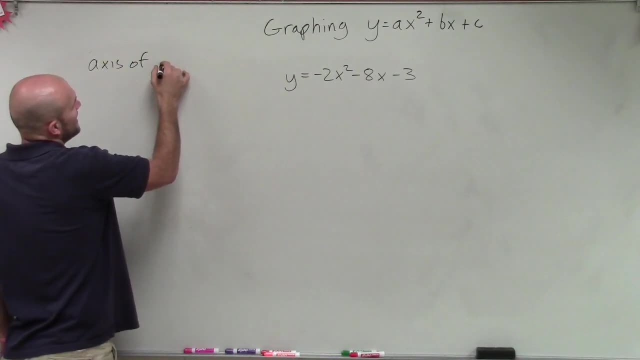 we'll use the axis of symmetry to reflect over the axis of symmetry to find our exact same coordinates. All right, So the first thing we need to do is, though, find our axis of symmetry. So our definition of the axis of symmetry is x, which is a vertical line. 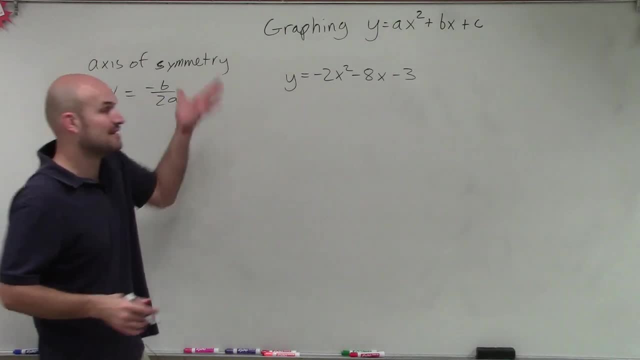 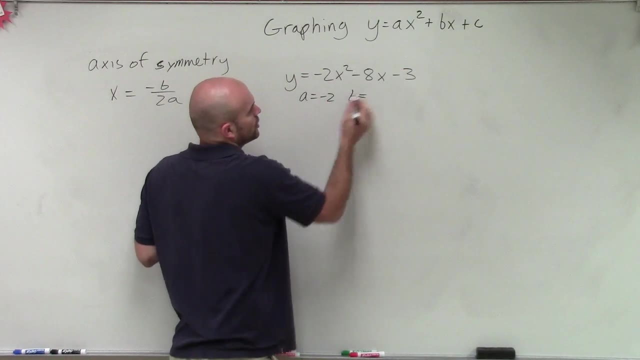 and x equals. So x is the opposite of b divided by 2a, which is going to represent a vertical line. Well, in this case we need to figure out what b and a are. So remember: a is our coefficient of our quadratic term, b is our coefficient of our linear term and c is going to be our. 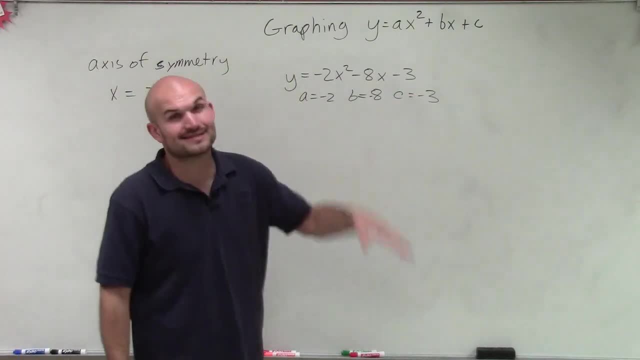 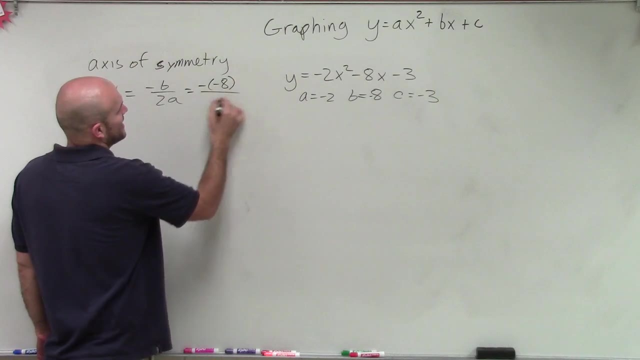 constant. Now we're not going to use c for the axis of symmetry, but it's kind of good just to know. So therefore, we have: opposite of negative 8 divided by 2 times negative 2.. Notice, it's opposite of b, Since b is negative. it's opposite of negative, which. 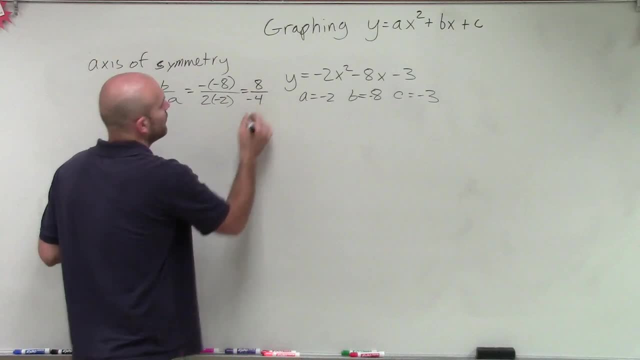 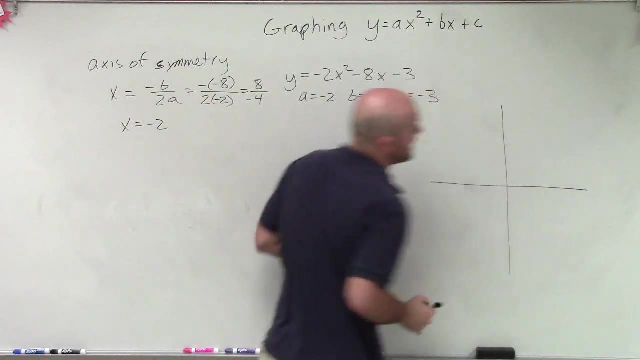 is now going to make this a positive 8 over negative 4.. So therefore, my axis of symmetry is: x equals negative 2.. So now on my graph, I'm going to go over and I'm going to plot my axis of symmetry, which is at negative 2, which is going to be a nice little vertical. 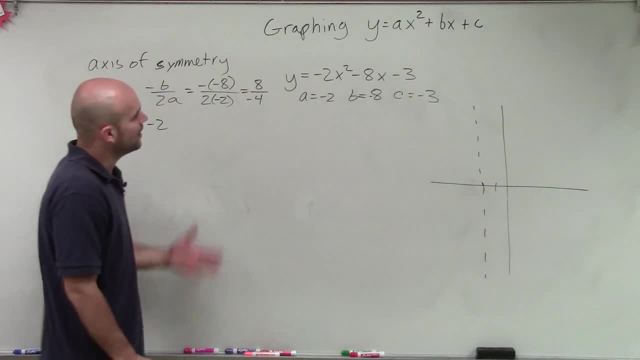 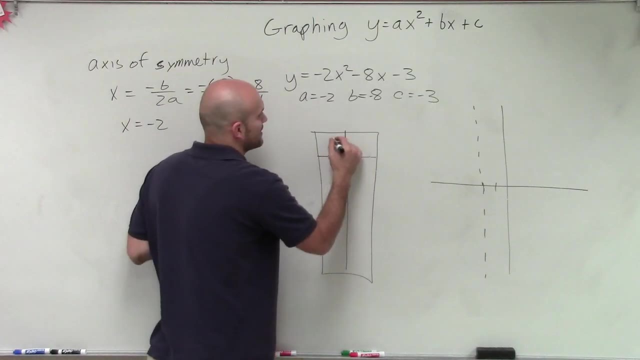 line. So we can say that x equals negative. 2 is right there. All right, So now we need to choose our table of values Now in before. what I have done is I have always chosen two points, to the left and to the right, And the reason why I did. 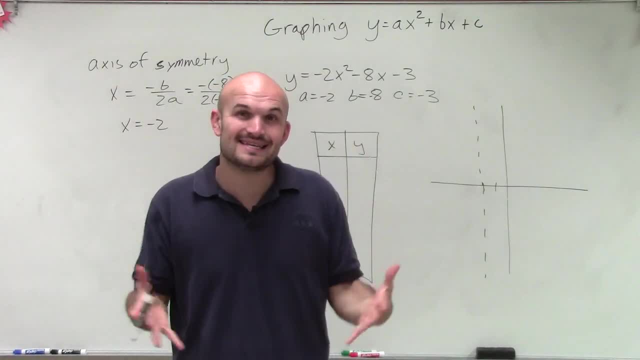 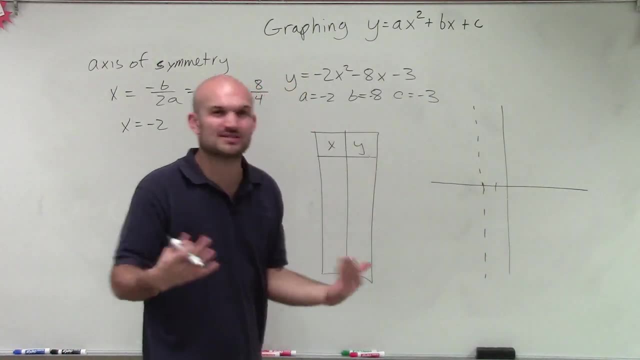 that is because we wanted to make sure- and also for you guys to see- that our points to the left and to the right, the y-coordinates, are exactly the same. And that's so important, because now we don't have to always do all that legwork, especially when we have a problem like this. 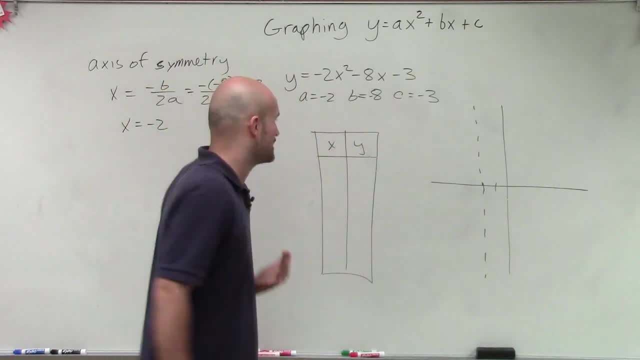 where we're going to have a lot of math involved. It's a lot of work to keep on adding all those values. So if I say my axis of symmetry is at negative two, then all I'm simply going to do is let's just pick two points to the left, Or you could pick two points to the right, but a lot of 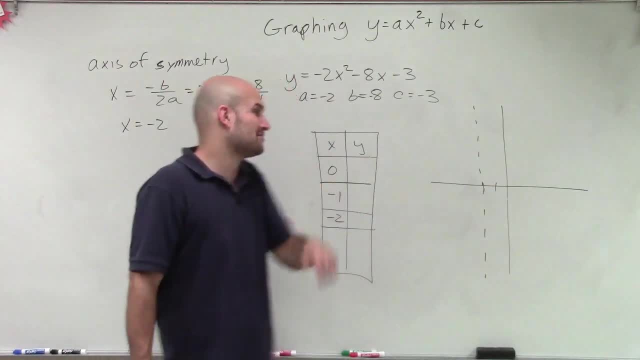 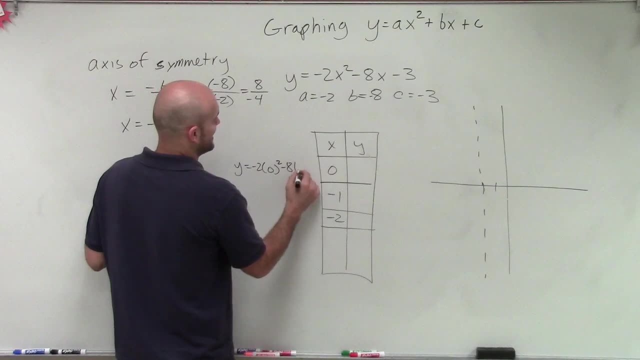 times. I like to maybe keep it, you know I like where zero is in one. Those are good numbers to use. So now let's evaluate for: y equals negative two times zero, squared minus eight times zero minus three. Well, zero squared is zero times negative. two is zero minus eight times zero. 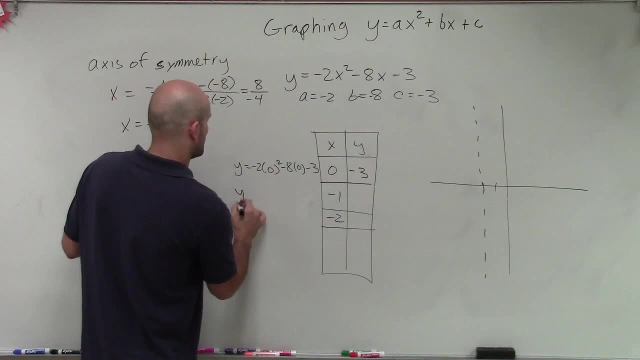 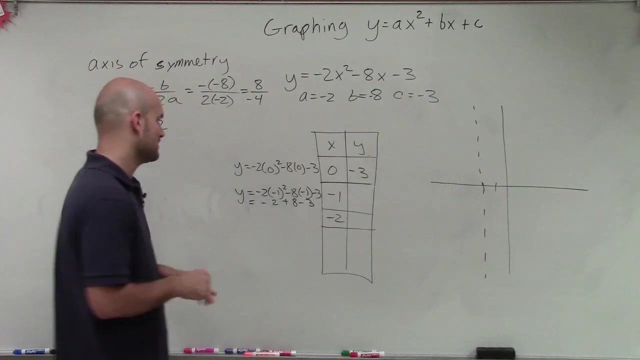 which is zero negative three. Then let's do one: Y equals negative two times negative, one squared minus eight times negative one minus three. So therefore this becomes negative one negative one squared, So that's negative two plus eight minus three, So that becomes negative five plus eight, which is 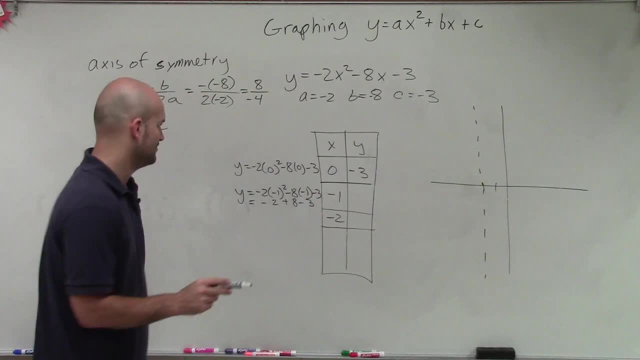 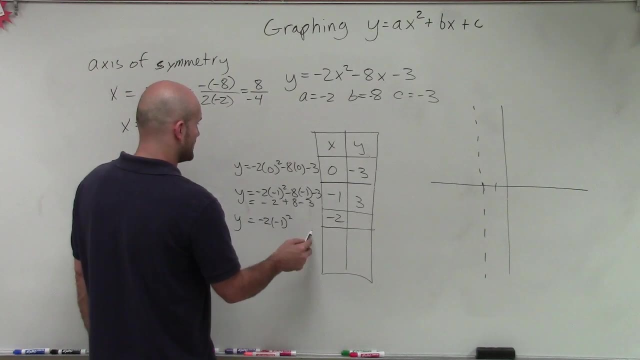 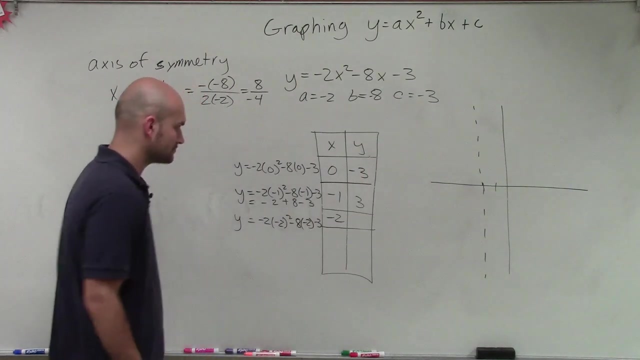 now a positive three, And then let's do negative two. Y equals negative two times negative one squared. We're going to do a negative two squared minus eight times negative two minus three. Oh, and let's go and pick my two points to the right. So if that's at negative two, then we'll have 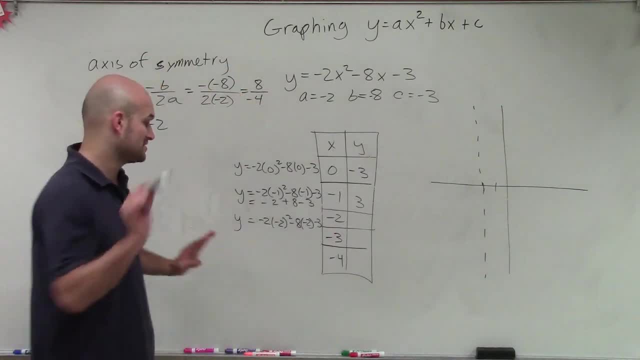 negative three and negative two. So that's negative two. And then let's do negative two and negative four. All right, I'm not going to evaluate for these. I'll show you why in a second. So therefore this becomes negative two squared, which is four, Four times negative. two is negative. 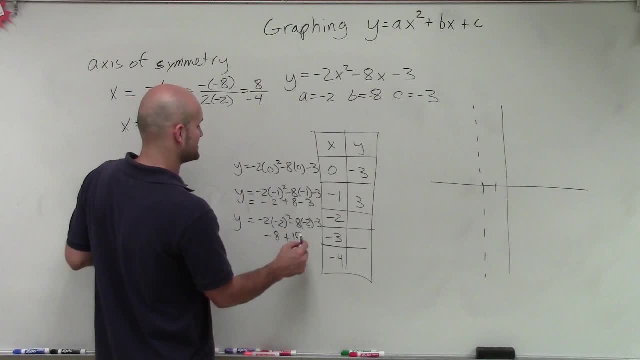 eight Negative two times negative eight is going to be a positive 16 minus three. So therefore, that's going to give me now a that's positive five. So that's going to now give me a positive five, All right. So let's go and plot these points and see what it looks like. So, at zero. 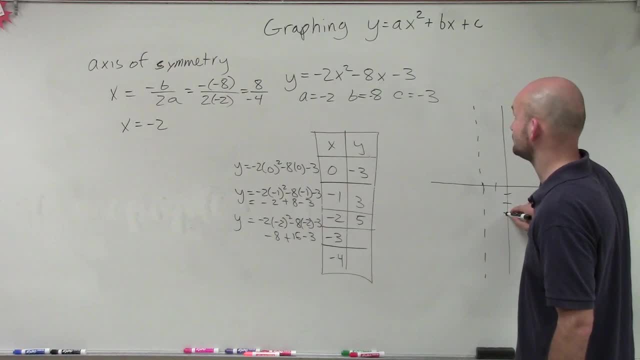 I have negative three, One, two, three. At negative one, I'm up at three, One, two, three, And then at negative two. I'm up at five, One, three, four, five. All right, So right. 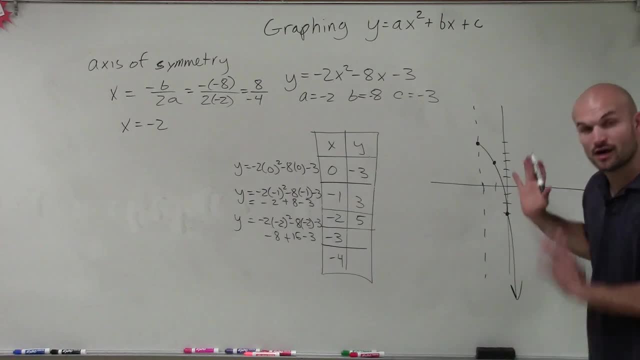 now I have a graph that looks something like this Right Now. remember, the axis of symmetry reflects our parabola, So therefore I know if this point is one away from the axis of symmetry. So if I go to my next point, which would be at negative three, I know that point. 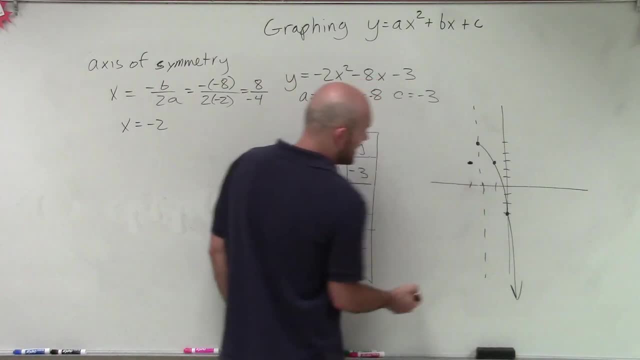 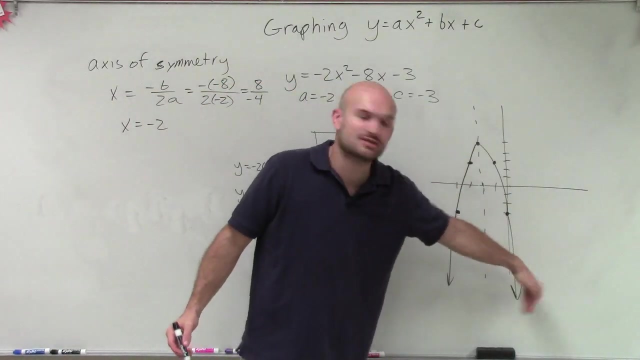 is also going to be three. Then if I go over two points and over at two points, I was down at negative three. So at two points over here, I'm also going to be down at negative three. And so now what you can see is, by using the axis of symmetry, I plotted points to the